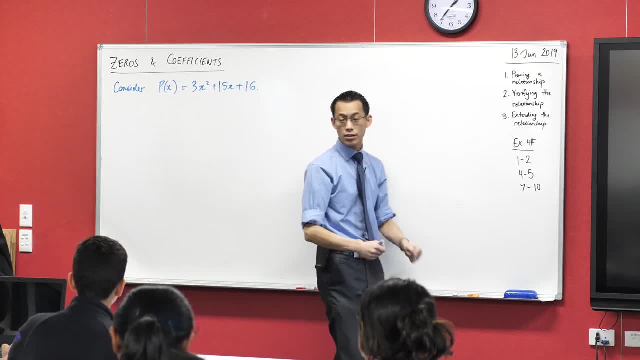 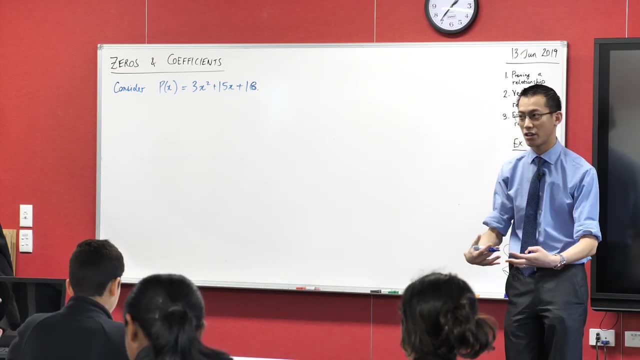 this with some brackets and all that kind of thing. is there anything simple we can do? oh sorry, that number on the end should be an eight. that's an eight. Is there anything simple we can do to make that factorisation a bit simpler? Yeah, each one of these numbers. that's why I noticed my 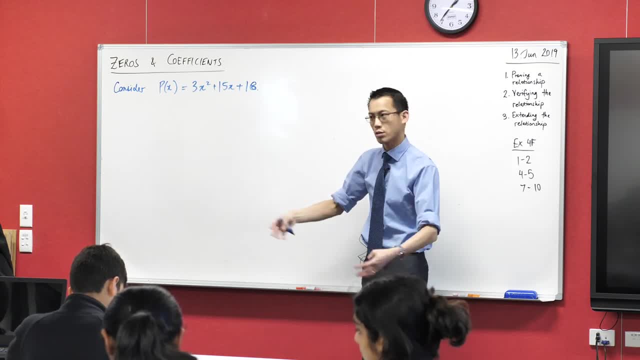 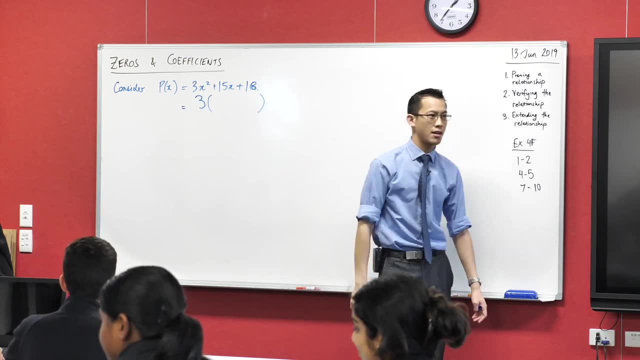 number was wrong. each one of these numbers is a multiple of three, so I can just factor that out. let's do that. So I'm going to write out the front: a three. and what does that leave me with on the inside of the? 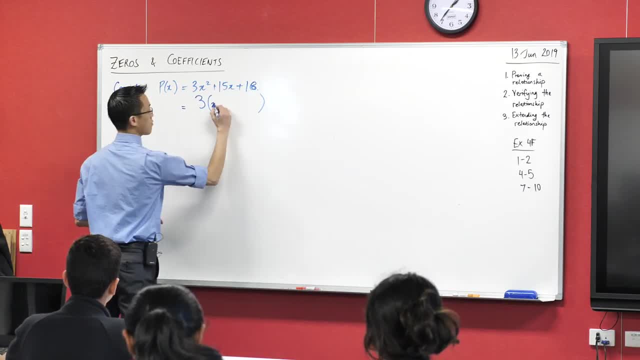 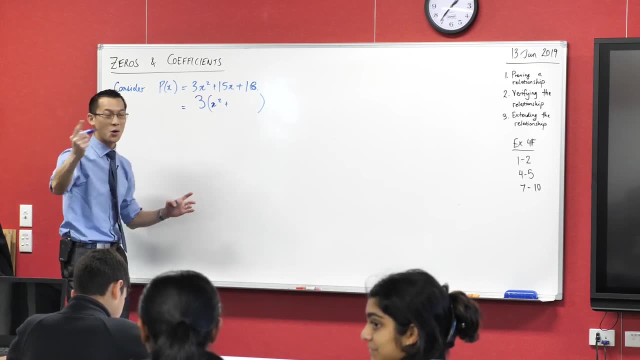 brackets. Okay, I got an x squared. someone take over. what's next? Someone who just walked in- you can see this- tell me what's next. Come on, you guys can all see this. what's my next term? 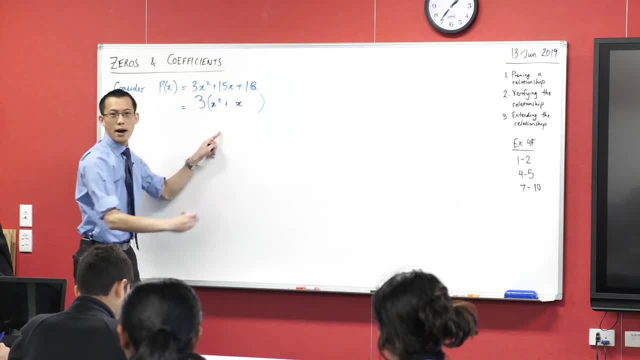 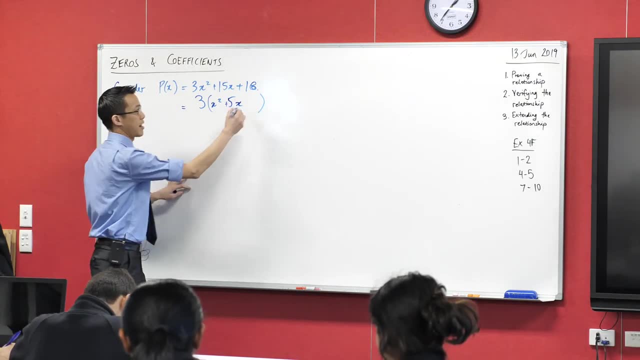 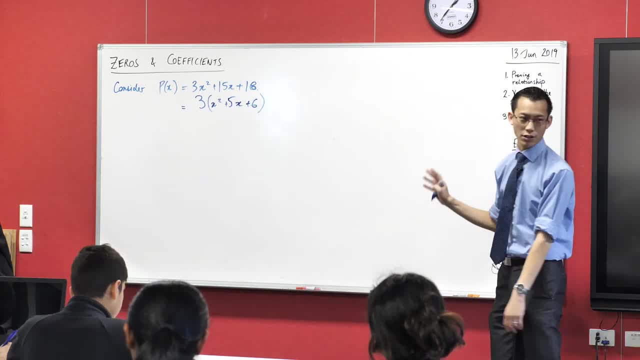 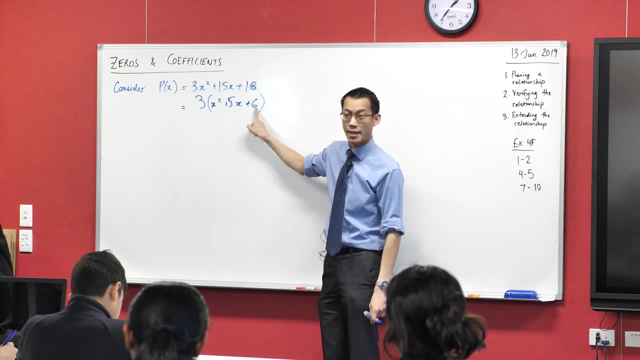 we've taken down a common factor, And now, when you have a look at this thing, you can see why I chose these numbers. These are really easy to deal with, right? We're searching for a pair of numbers. Add to that, multiply to that In those two numbers, of course. how interesting. so I am. 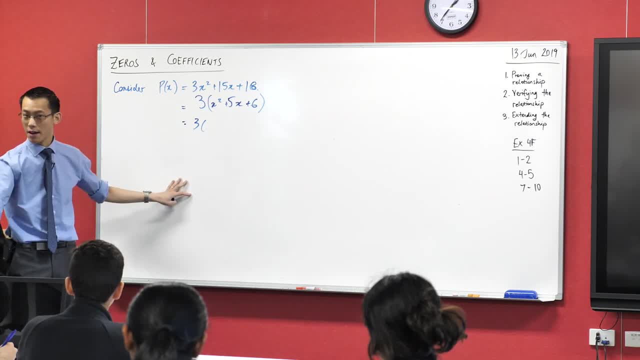 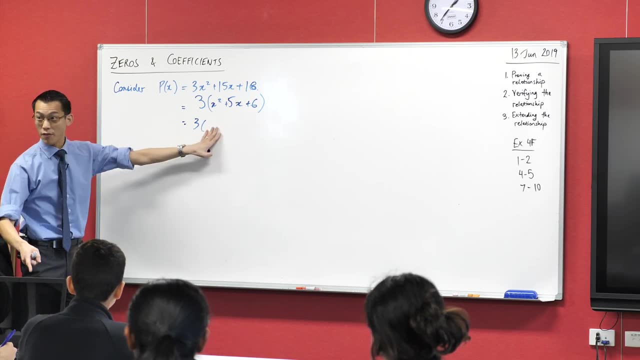 going to write eventually, minus 2 and minus 3.. But those are not the factorization. You're actually going to the next step, Serene, when I'm just doing the factorization, I'm not minus 2 and minus 3.. 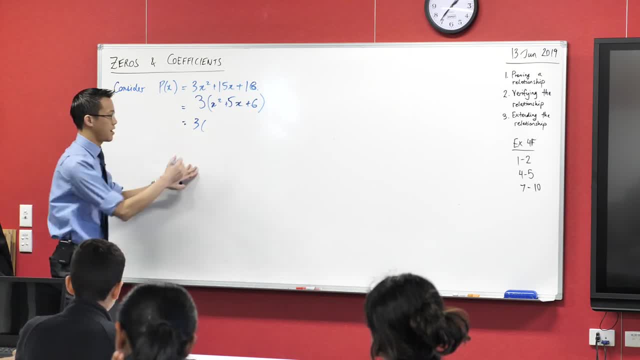 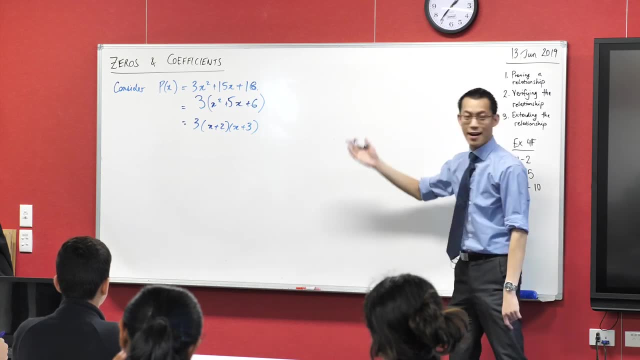 The numbers I want are plus 2 plus 3- right, I'm going to write my factorization like so. and the minus 2 minus 3, where they come in, are they are as the heading suggests to you. they are what we call the zeros of this polynomial. this is our polynomial p of x. 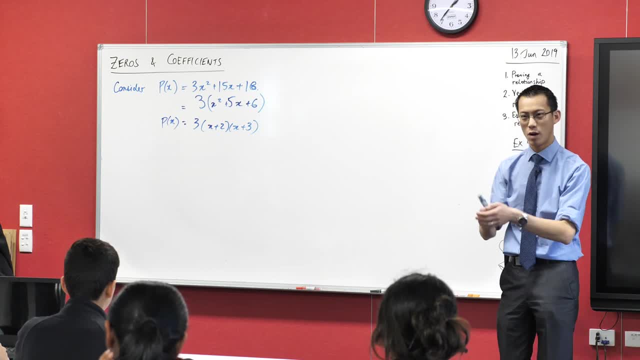 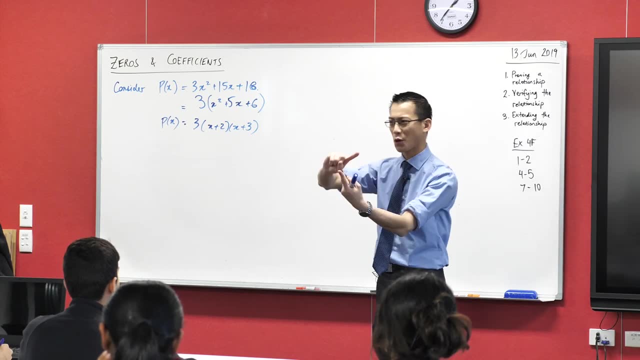 why do you think zeros? remember, we've talked about this language before. why do we call them zeros, minus 2 and minus 3? what happens with them? yeah, they, they are the x intercepts. we've talked about x intercepts, we've talked about roots and we've talked about zeros. I want you to look again at the web. zeros, it's a. 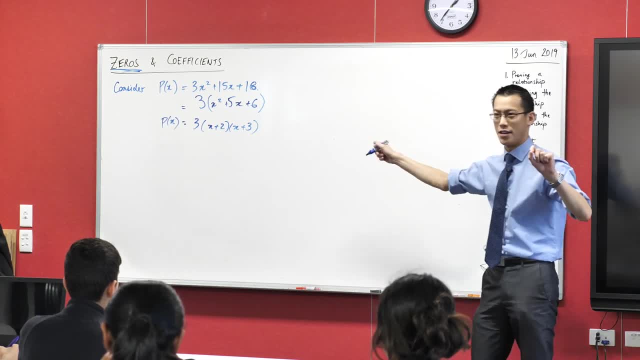 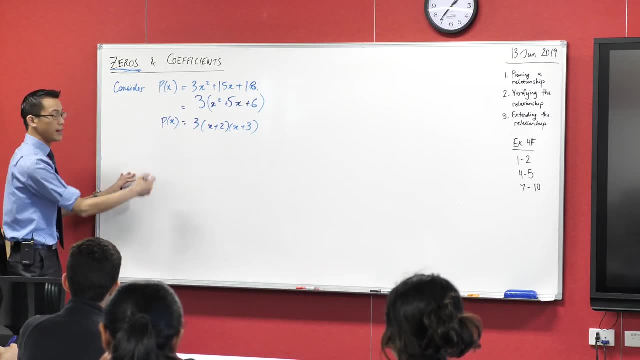 bit weird to say negative 2 is a 0 of this, but why would that actually be a sensible name? wrestling, they make the whole thing 0. please mark that right. let's actually write that down. I'm going to put it in different color just to. 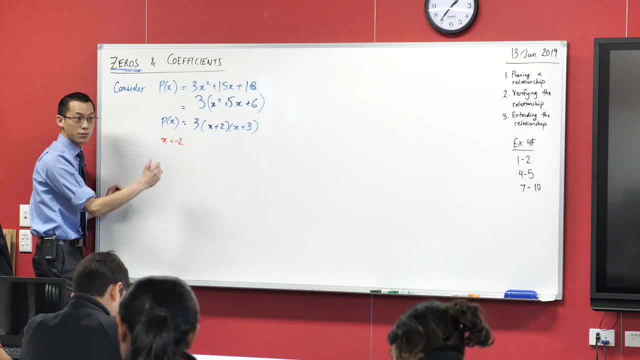 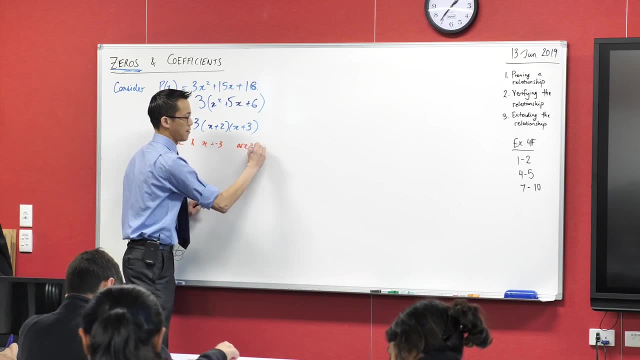 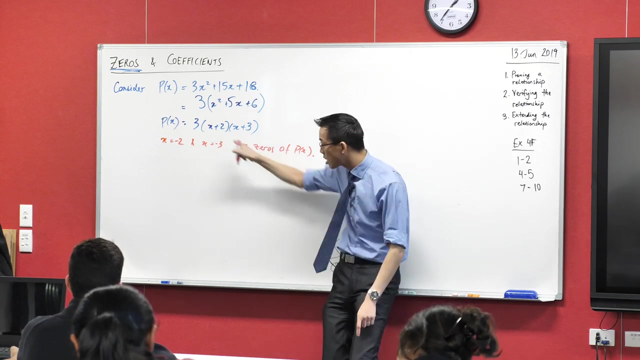 highlight it right, I'm going to say: x equals negative 2 and x equals negative 3 are zeros of this polynomial, right. right, they are zeros of p of x, because if we took negative 2 and negative 3 and substituted them in p of negative 2, p of negative 3, then you get 0 out of this. 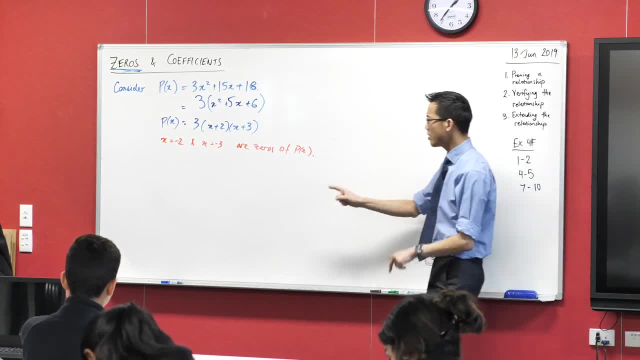 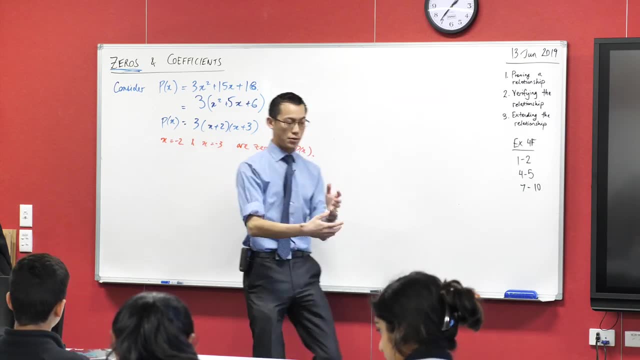 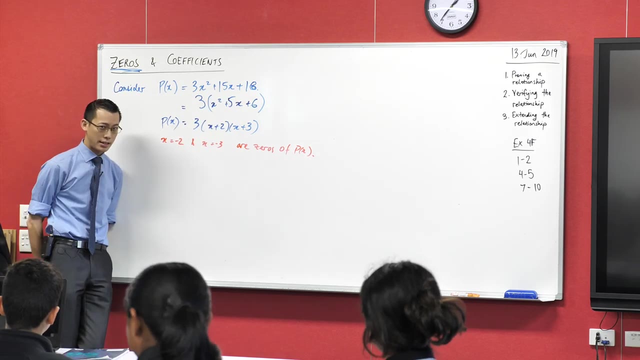 that's why we call them that. okay, now, these two numbers here- negative 2 and negative 3- I wonder if you can see there is a relationship between these two that you can get straight out of here without doing any of this factorization. let me see if I can tease it out for you a little more. 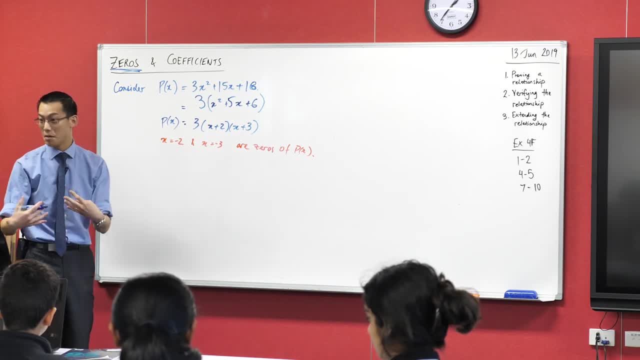 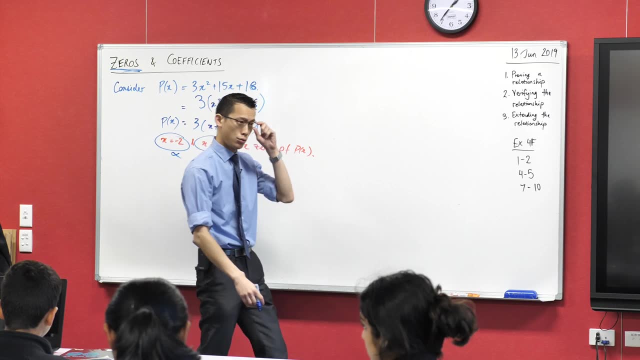 let's give these two x equals negative 2 and x equals negative 3. let's give them names. well, let's call this guy over here alpha and we'll call this guy over here beta. these are my two zeros. I'm gonna ask you to do two things with them. number: 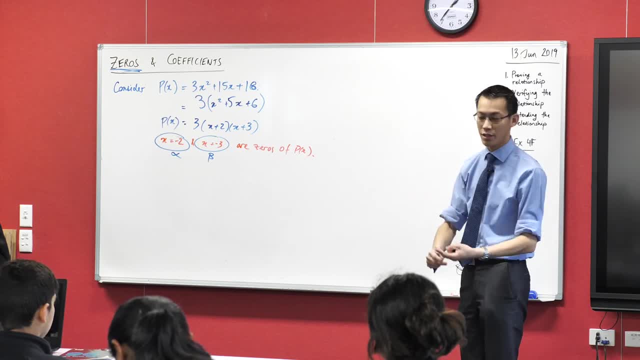 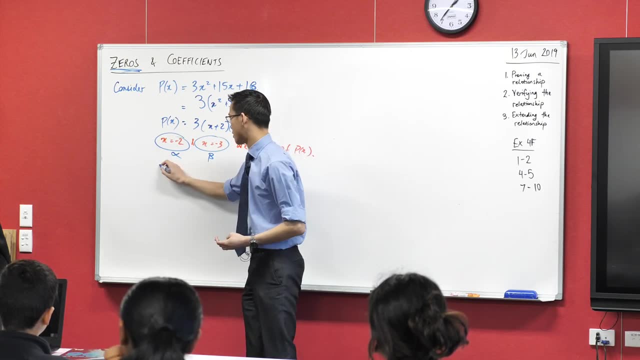 one. we're going to add them up, see what we get, see if there's anything interesting. then we're going to multiply them, see if we get anything interesting. okay, so to add them the way I would write that: the sum of these two roots I'll write that as alpha plus beta, right? 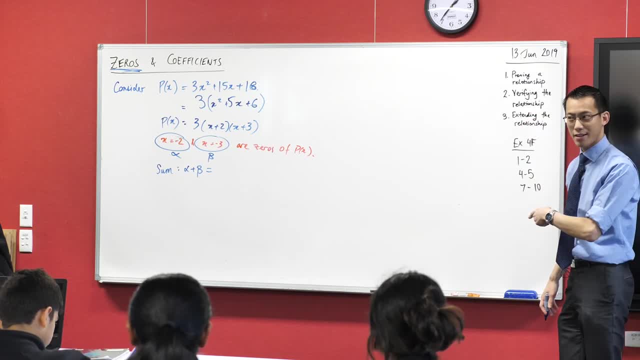 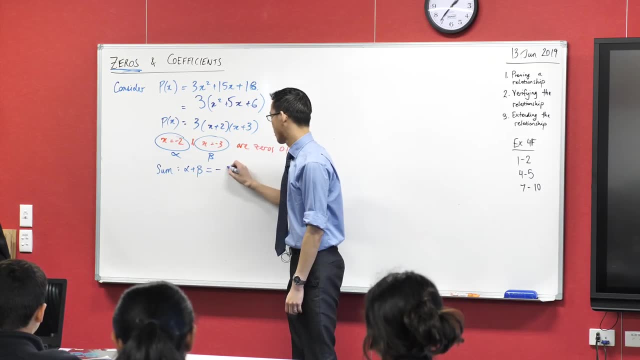 there we go. when you take a particular value, is Alvin Bear negative 2, negative 3- you add them together, we get, of course, negative 5. okay, let's just hit pause on that guy. and then the other thing I wanted to do was multiply them together. 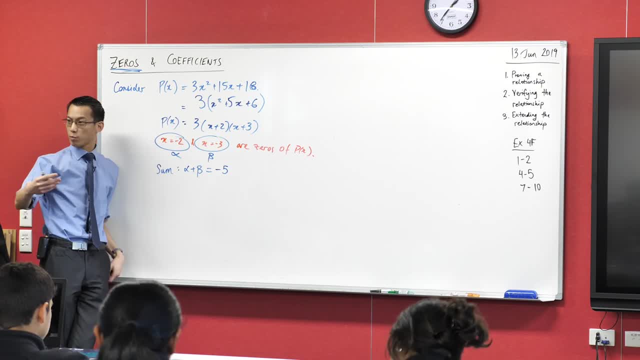 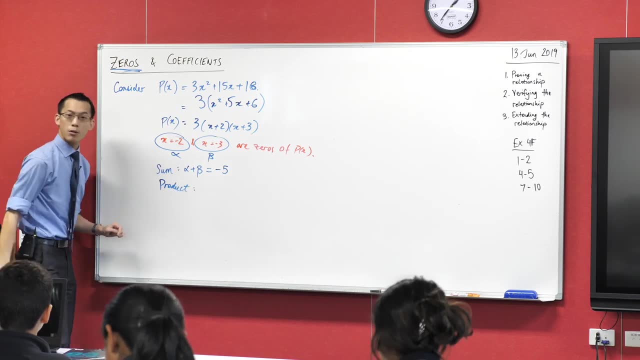 that's not a sum. what happened? what's the? what's the answer called when you multiply two things together, it's a product. right, it's a product. that's what happens when we multiply two things together. so I would write that as not alpha plus beta, but alpha times beta. 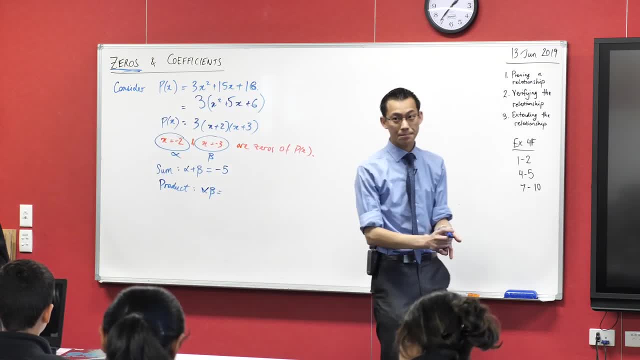 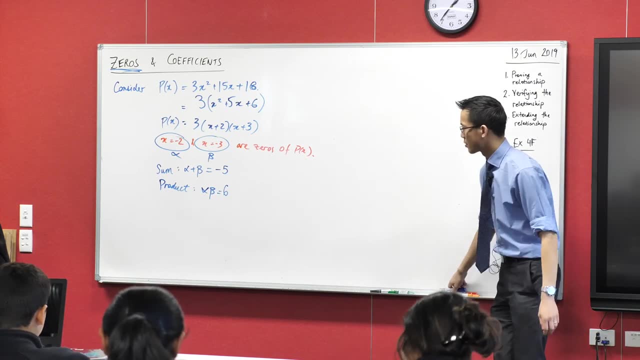 I'm just going to leave out the times. What do you get? What's the answer? It's 6, right, Okay. Now I wonder if you notice there is a clear relationship between these two numbers that you've gotten out here. 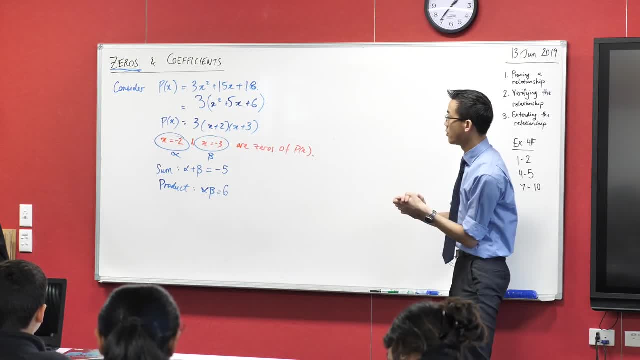 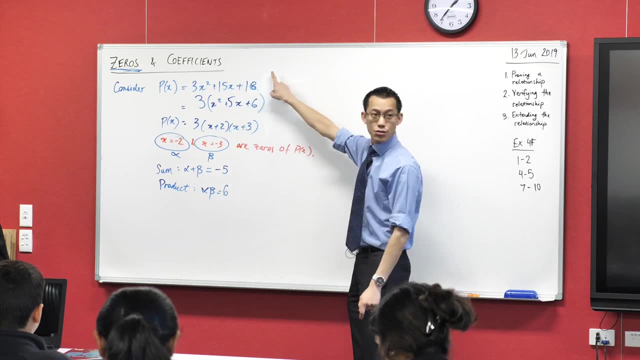 and our original, the first line of this, our polynomial right, And there's relationships all the way through. There's a relationship from these guys to here and also these guys to here. Let's start with this line. It's a bit easier to see. 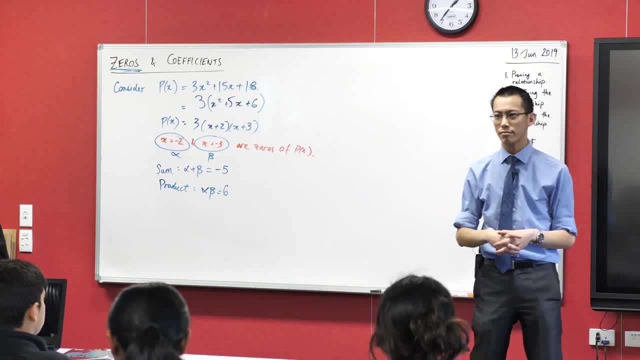 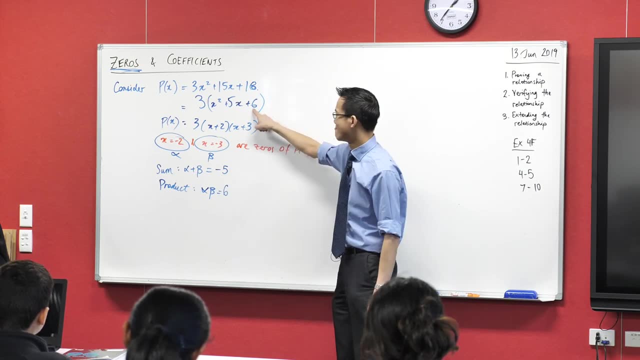 Where do you see 6? Like, where do you see it? It's just the constant term. It's just right there, isn't it right? There's 6.. Where's negative 5? That's a little trickier to see because it's negative. 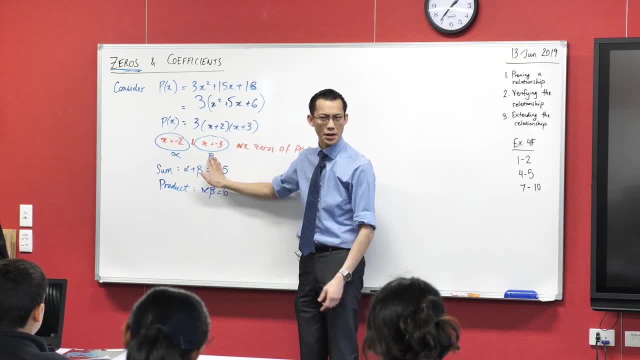 Maybe I should ask: where's this guy? Where's the 5?? We have language for this, right? It's the coefficient of x. Thank you right, It's that guy right there. So where do we see this? It's the negative of the coefficient of x, right? 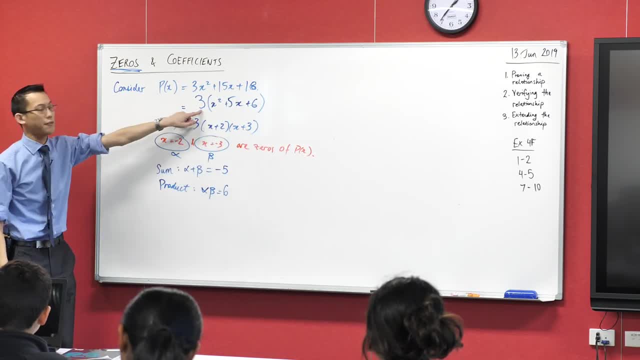 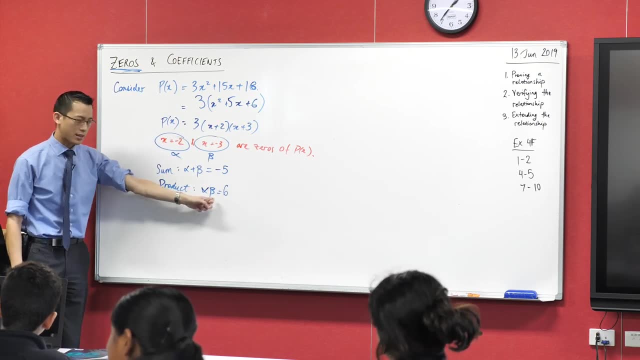 Hmm, But to get to this line, what we had to do first was we had to factorize out. Do you see that We had to take out this factor? It went all the way through, okay. So in fact, how can we get 6 and negative 5? 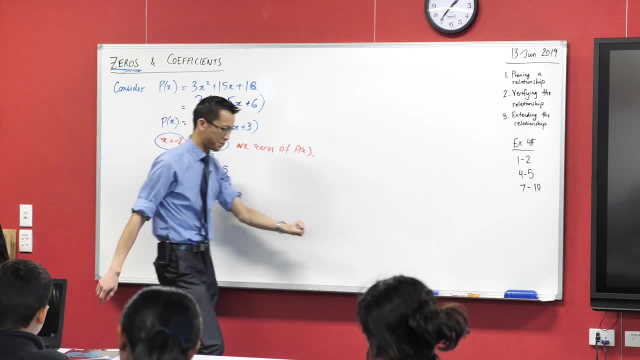 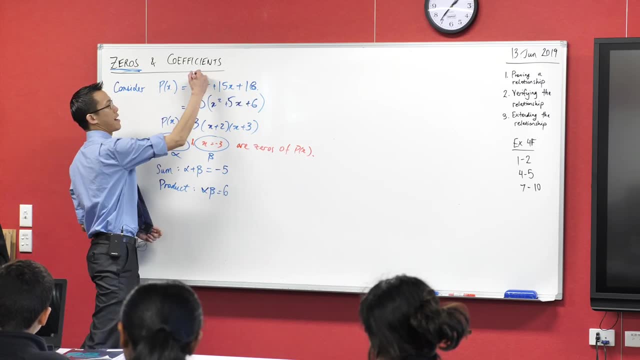 just out of this very first line. Well, this is an appropriate call. We're going to take that thing right down the end. When we look at this quadratic, we would normally write it as this: ax squared plus bx plus c. That's the general form. 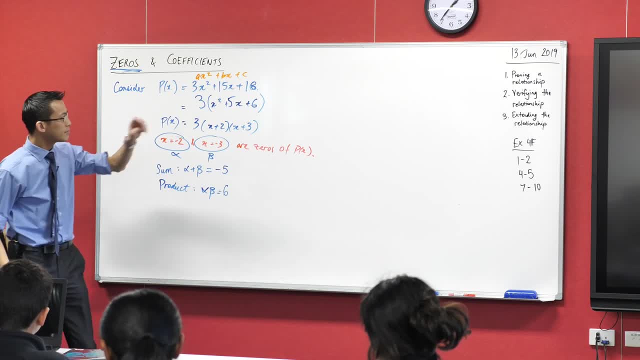 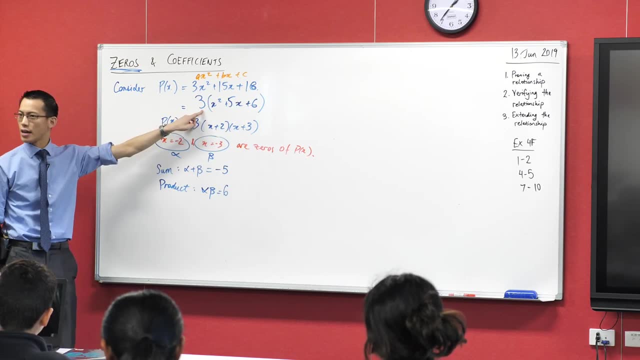 You can describe any quadratic you like in this way. right? We took this last number and when we get to 6, to factorize out: I. well, I divided, didn't I? I divided by whatever this coefficient at the front was right. 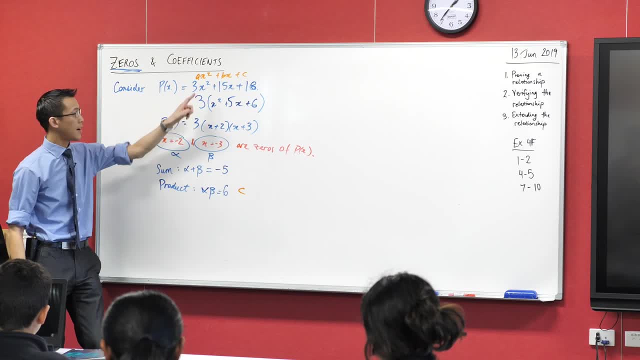 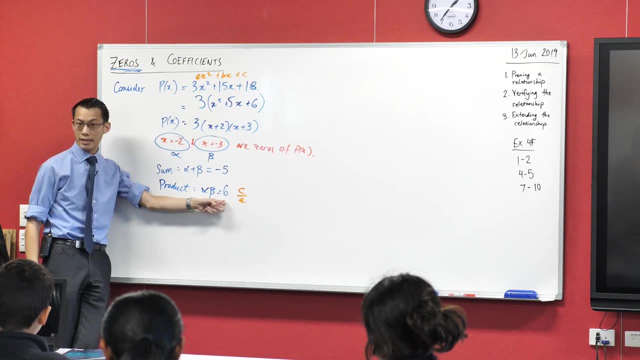 So I took c and then I divided by this coefficient at the front a. Are you happy with that? Do you see that? that's where I could get 6 without having to factorize. I could go straight to this value if I were so interested in it. 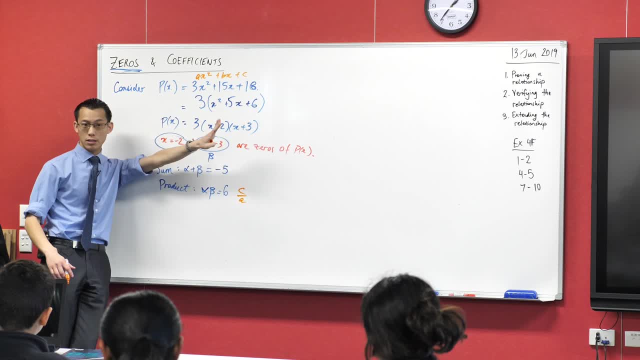 Is that all right? When you have a look at this one? I didn't look at that last term, I looked at the middle one, the coefficient of x. So that's not c, That's b, That's what we call it, right. 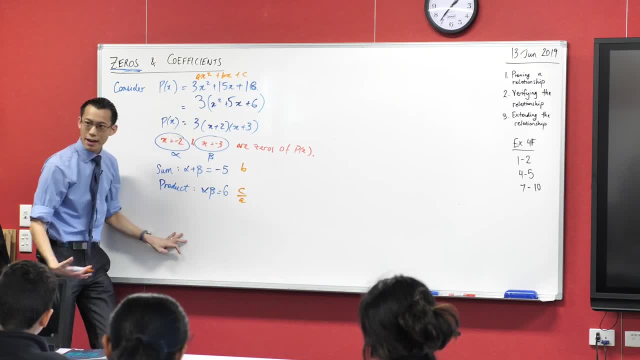 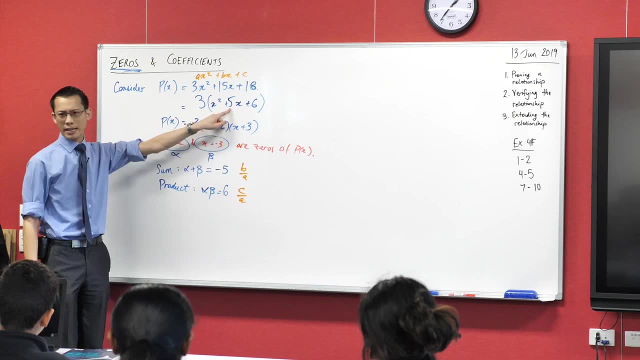 The coefficient of x. right there It's b. I factorized out. So again, just like here, I divided through by a. But then there was one last thing. You're like, oh, you don't get negative 5 here.